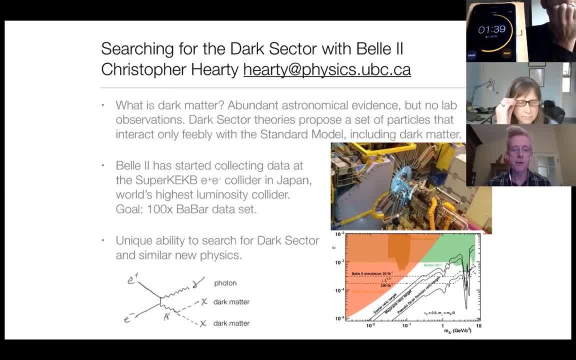 the gist of what's going on here. So we have a electron, a positron. this gives a photon and a hypothetical particle called the dark photon that would decay to the dark matter. So the only thing we can observe in our detector is the one photon. This is an 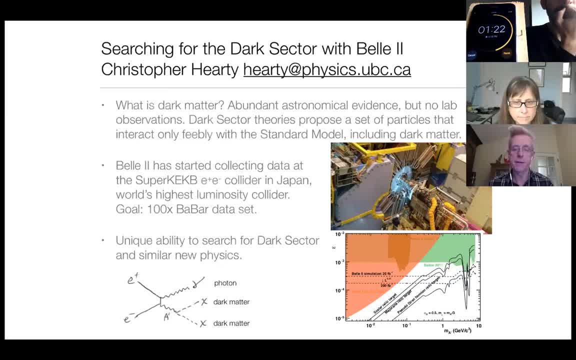 example of the type of analysis that we could do with our data set. What gives us this unique capabilities are the features of the E plus, E minus collider, where it's a very clean environment. It's also the fact that we are going to get a 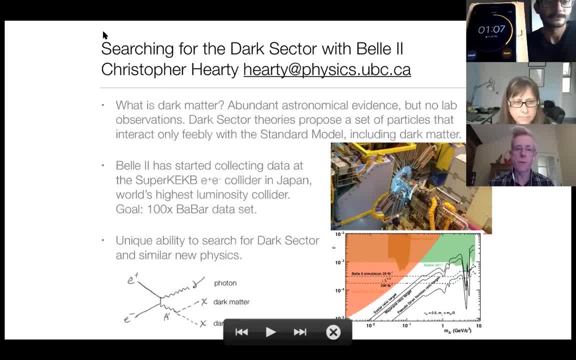 tremendous amount of data. Our goal is to get a hundred times what we collected. in the last experiment we did like this, which was called Babar. This diagram on the bottom right here gives predicts where, in parameter space, in these parameters of this model, the theories, the parameters have to exist to explain. 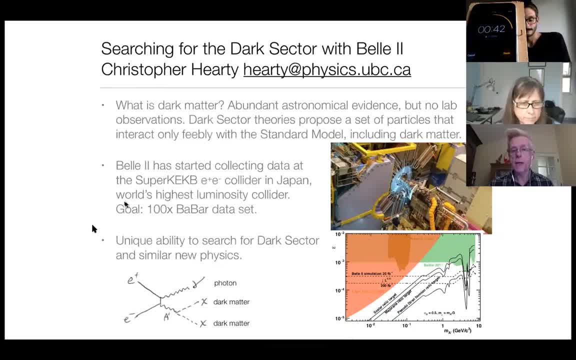 the astronomical dark matter. And the point is we have access, that we should be able to reach these part of the parameter space. So, in other words, if this theory does explain dark matter, we should be able to see it in our experiment. So this is just one example of the type of physics I do, but this 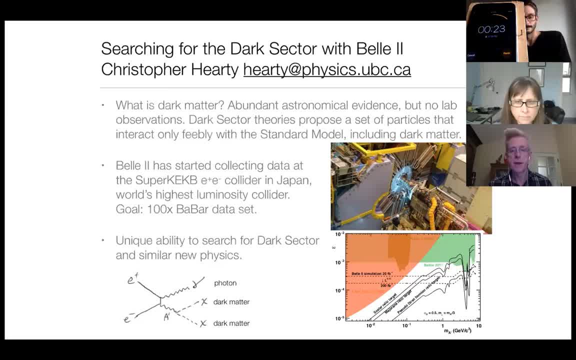 direct search is for new, new physics. It's a good time to join. We've just started taking data, So if you're interested, please get in touch. 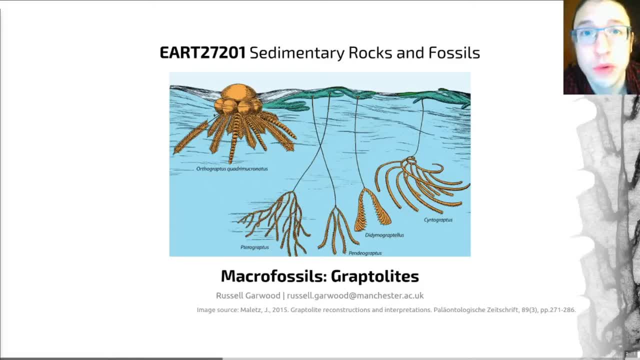 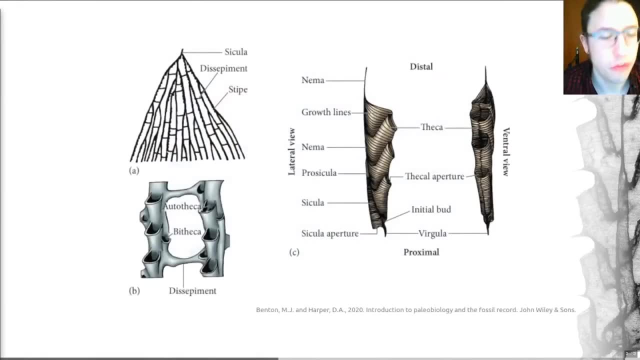 Hello everyone, and welcome back to video number two of Graptolites, in which we're going to be looking at the morphology of these animals. So let's start off by introducing the general elements of their morphology, irrespective of the group to which any individual Graptolite belongs.